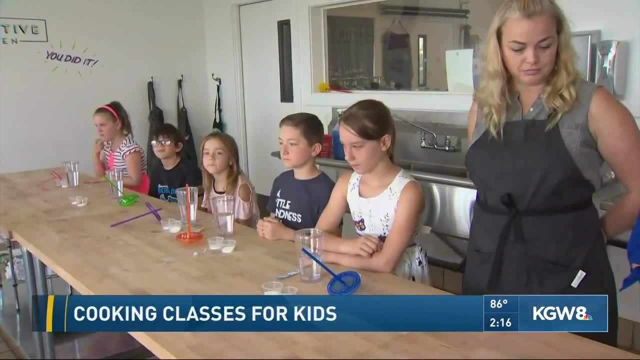 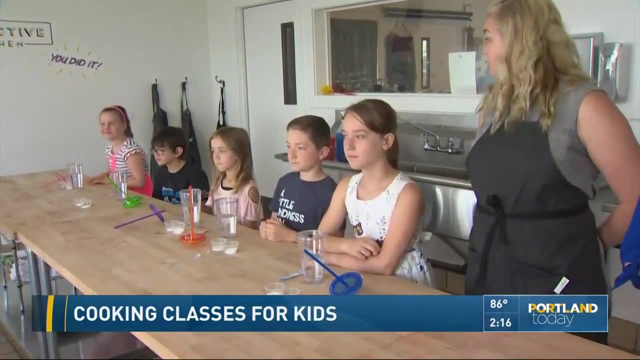 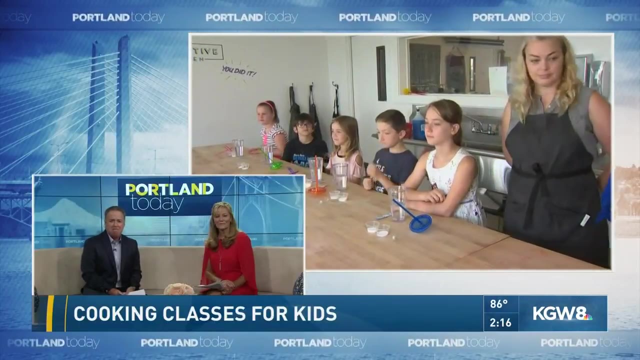 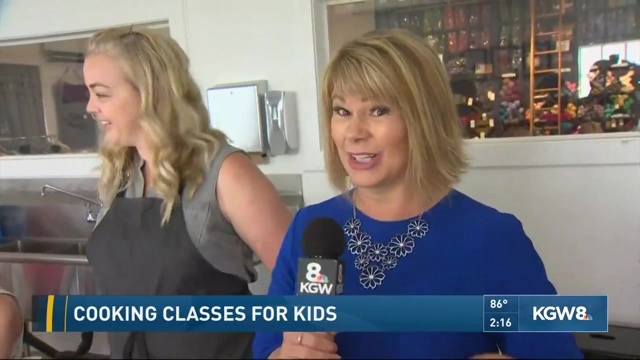 Some fun cooking classes to round out the summer for the kids. The classes have a strong science component. Yeah, so this is fun. I guess I didn't. I blew past that. I just saw the word cooking and I thought food. But Tracy, you're answering all types of chemistry type questions for us. Super fun classes coming up for kids. We're here with Shannon Feltus of Urban Farm Foods. We're in Hillsboro at a really cool kind of cooking classroom setting. And, Shannon, what are these classes going to be like? 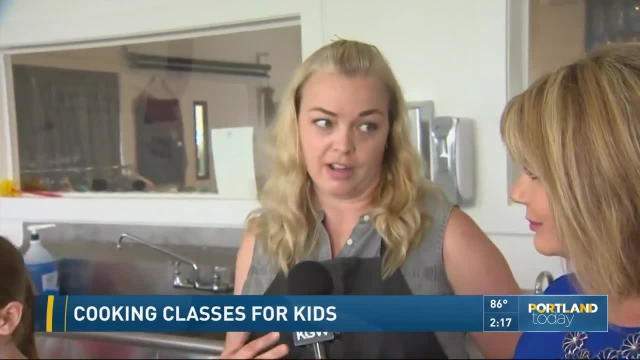 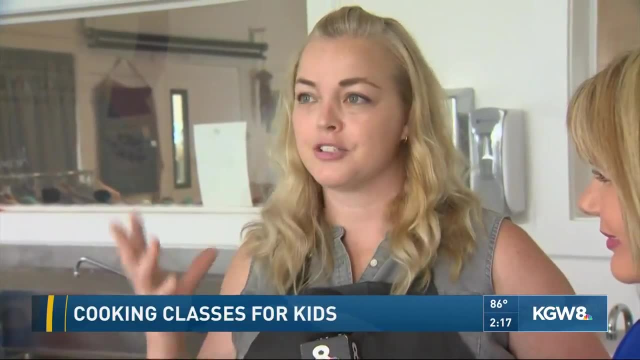 So Collective Kitchen has a lot of different classes And one of the ones that I'm offering is edible science for kids, And we make all kinds of things from soda pop and popcorn and edible Orbeez and things that are fun and tactile for the kids. 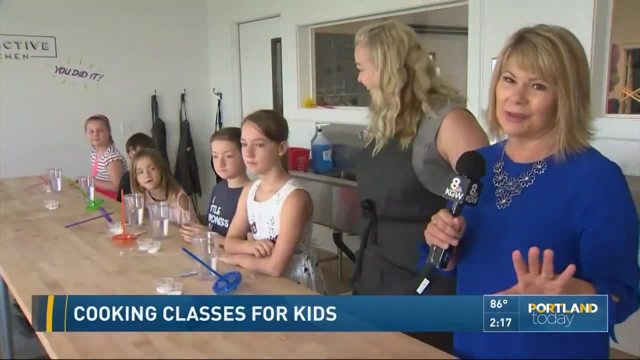 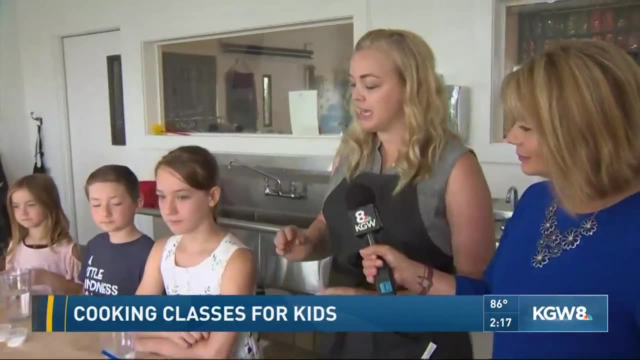 Okay, so we're going to make something today- Actually, the kids are going to make something. I'm not allowed to touch anything. You know how that goes. So, Shannon, what are you guys going to do? We are making soda today, So we're going to take key ingredients to make carbonation. 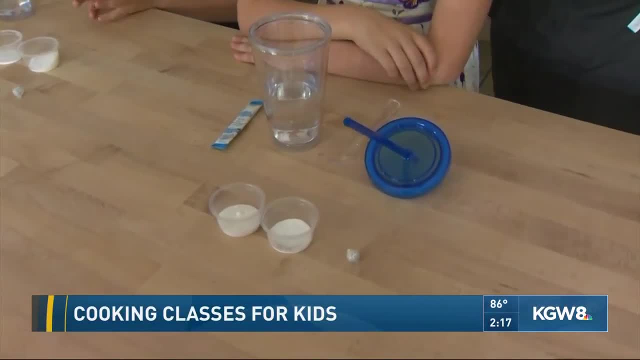 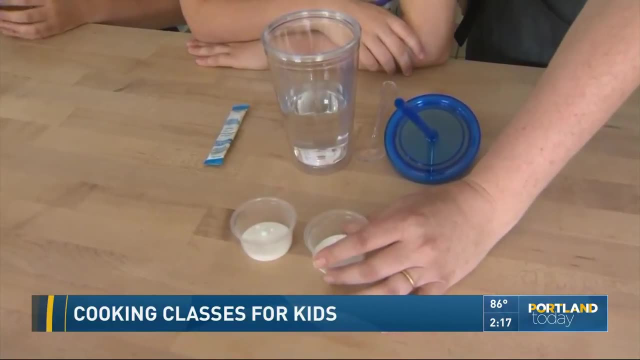 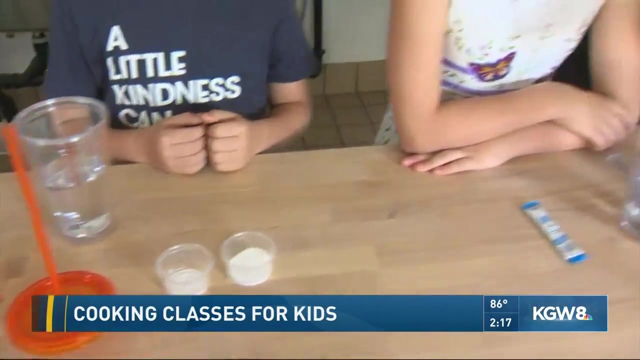 And then we're going to add a little bit of soda. Okay, go for it, All right. So you guys, in front of you you have your water and your two secret ingredients, that are baking soda and citric acid. So when I say three, you're going to dump these two into your water and we're going to see what happens. Are you ready? 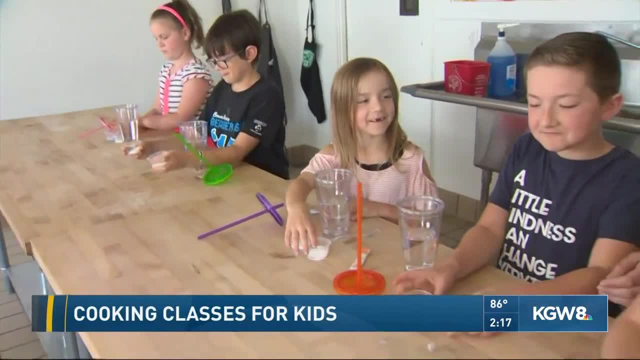 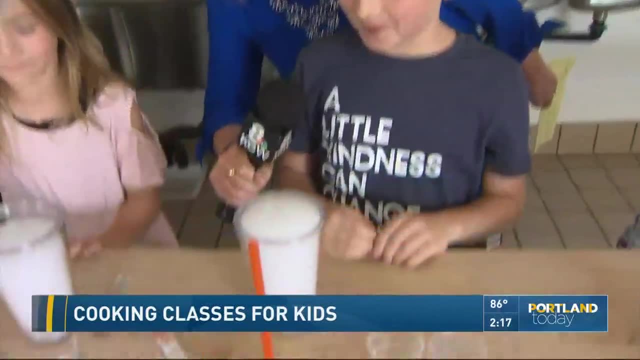 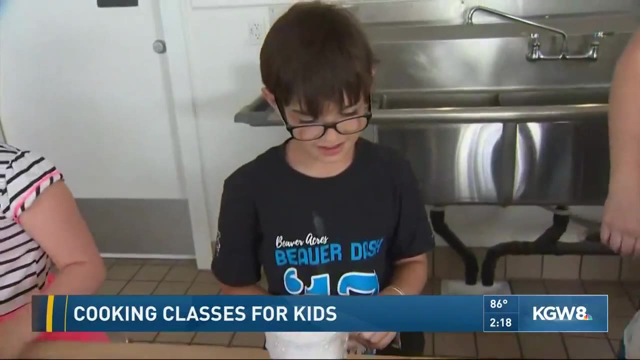 Okay, one, two, three, Go for it. Oh, what's happening? What do you think is happening? It's going to explode, It's bubbling, It's going to explode everywhere. Oh no, Okay, this is a problem. I think we've had a terrible accident here, Rachel. 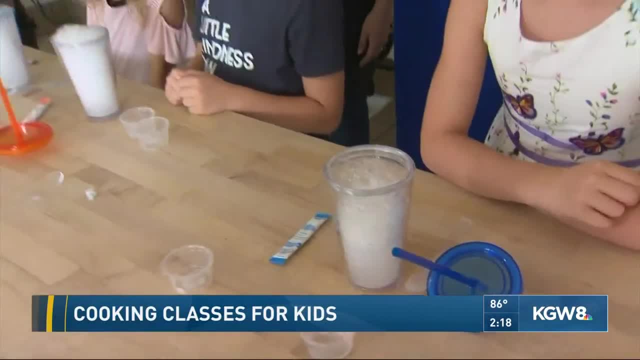 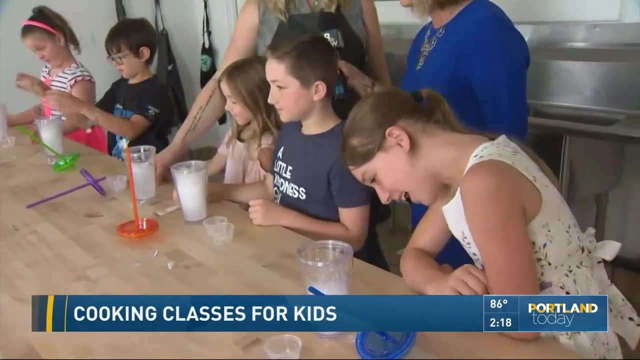 That is bubbly. So what happened? We've got paper towels, so it doesn't matter. We've got all the carbonation in our soda and now all we're missing is the flavor. Okay, So each one of these kiddos has picked a flavor, So you guys can open your flavor and add it to your soda. 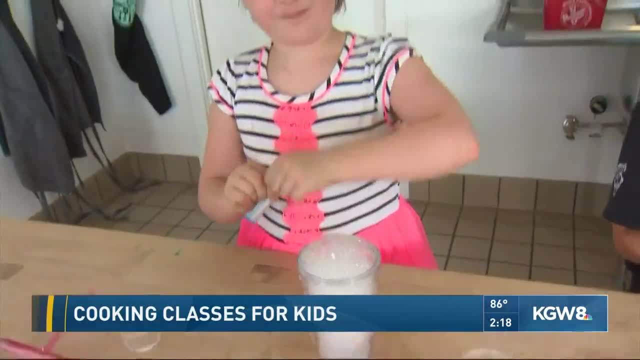 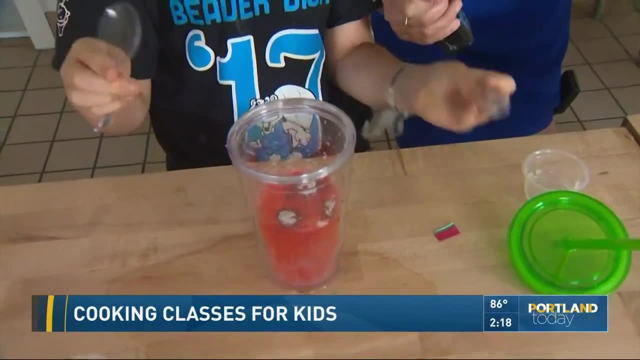 And then you can put your cap on and take a drink and see if you like it. Oh, I can't wait for the. Oh, I can't wait for the reviews. So what flavor did you choose there? Strawberry Crush? Oh, good choice. All right, Mix her up.